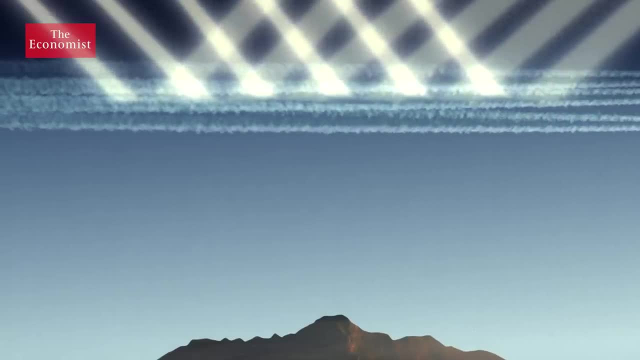 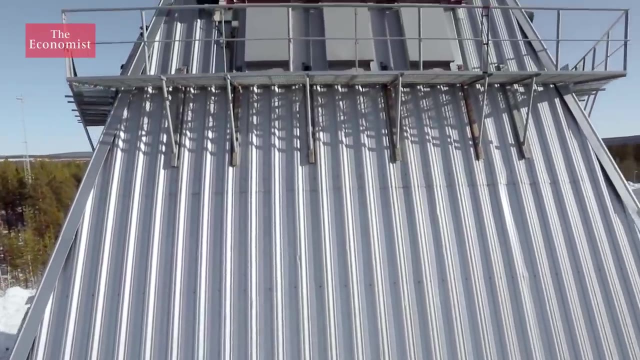 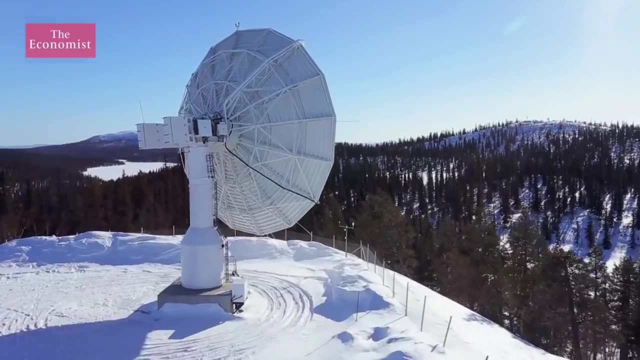 bouncing the sun's rays back. in the same way, In 2021, scientists from Harvard University researching solar geoengineering plan to test-fly a balloon from a nearby space center over territory where the Sami live. Ezra's testing area is in the mountain area. 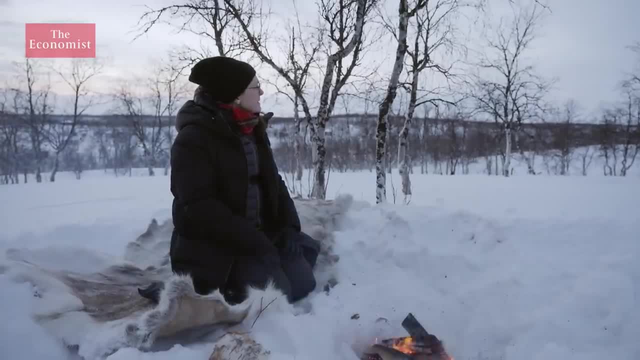 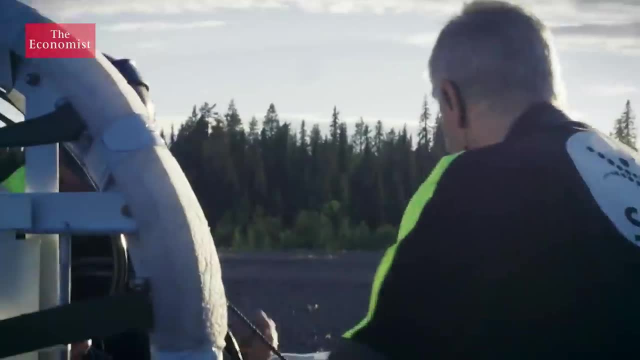 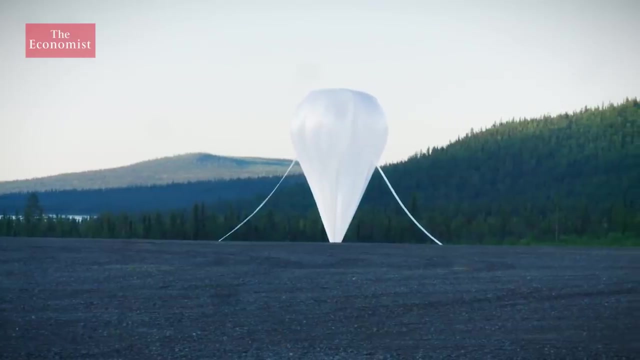 So this is the area where the testing would happen. The testing would have taken place Although the first balloon wouldn't have released any particles. a complaint from the Sami Council ensured it didn't take off and helped persuade Sweden's space agency to cancel the project. 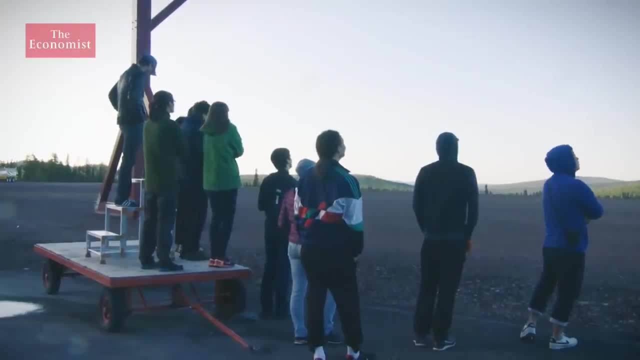 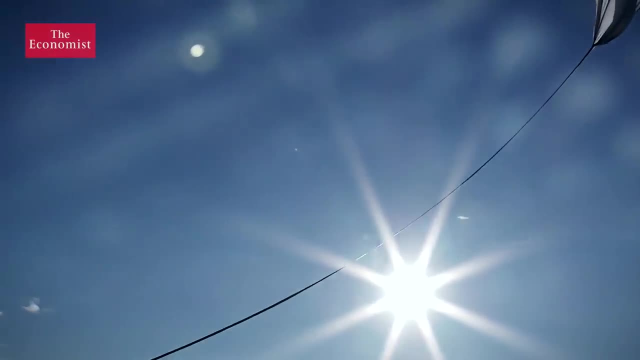 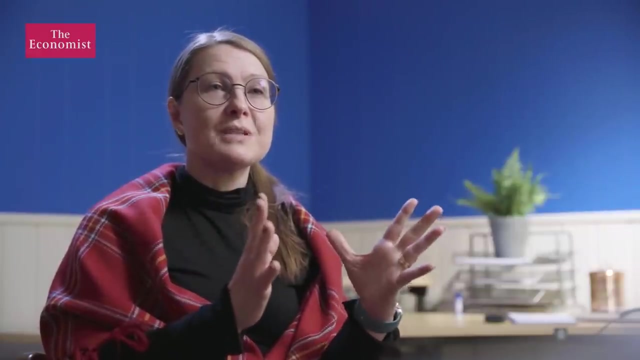 The Sami Council objects to the message this research project sends out about climate change. Like many, it worries that a successful technology would discourage the urgent need to reduce greenhouse gas emissions. The notion of a plan B, the notion of technology saving us. 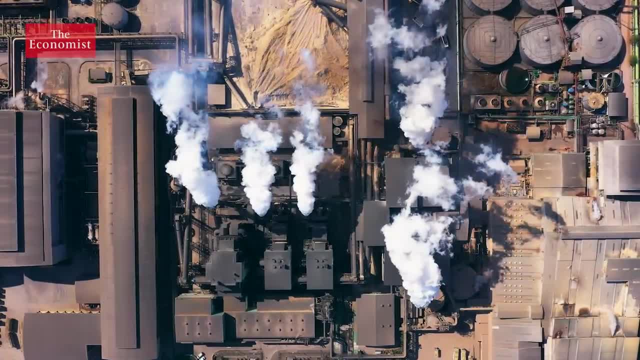 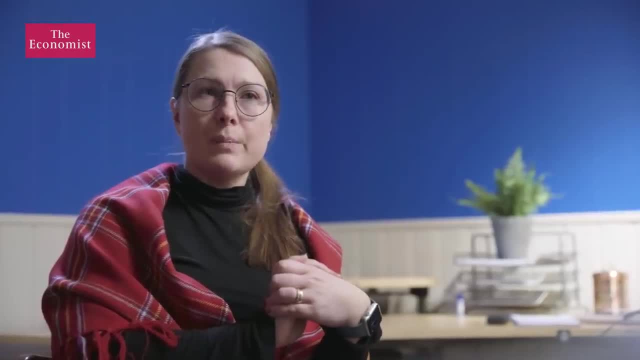 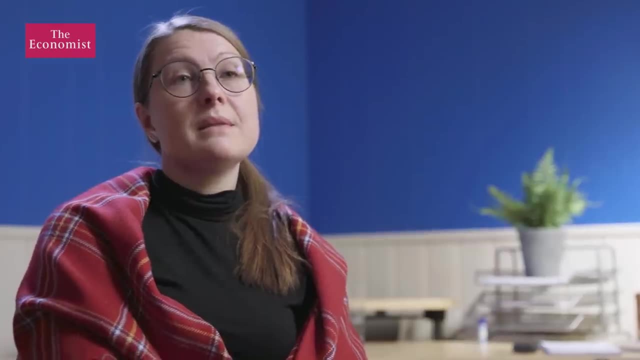 might put a pause on the needed climate action. If the fossil fuel industry leans back just a little and says, well, we'll wait and see a bit, just that notion might be the thing that makes us not reach the Paris Agreement, And that would be devastating. 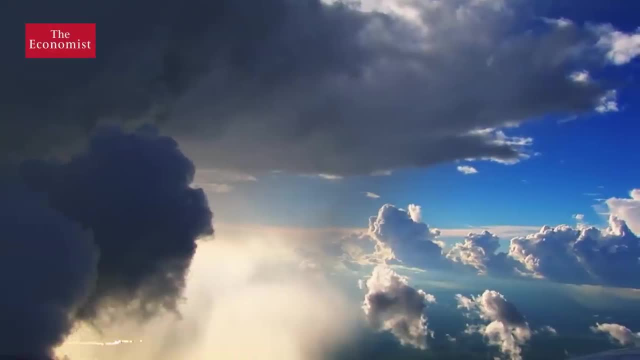 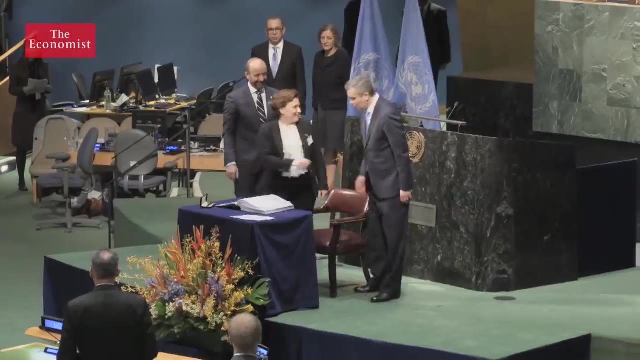 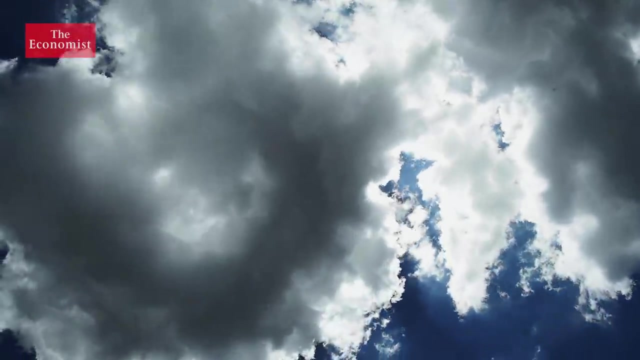 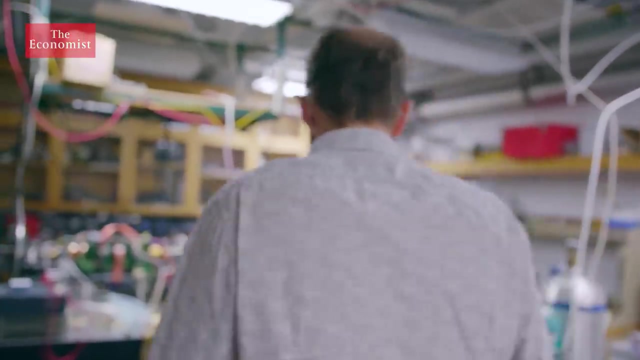 But models suggest that current political action is insufficient to limit global warming to the Paris Agreement's target of 1.5 degrees centigrade. So what about the case for doing at least more research into solar geoengineering? David Keith is one of the scientists in charge of the Harvard project. 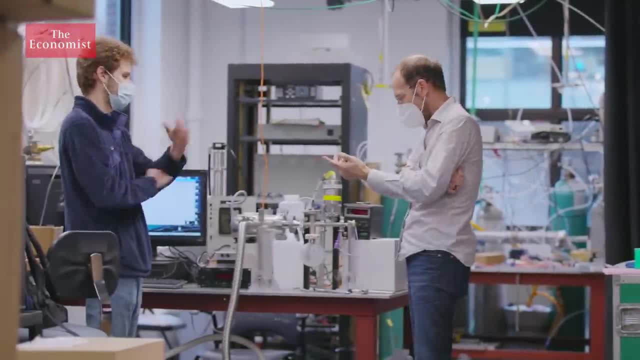 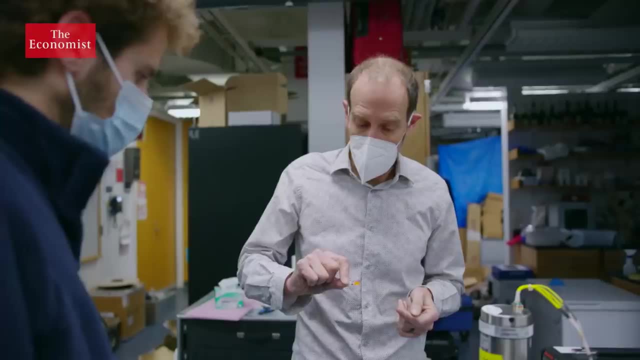 He argues, the risks from solar geoengineering must be weighed against the chance it could save millions from heat waves. Basically, your temperature noise is too big. The Sami Council are entirely within their rights to make a statement which effectively says that this whole line of research is unethical and a bad idea. 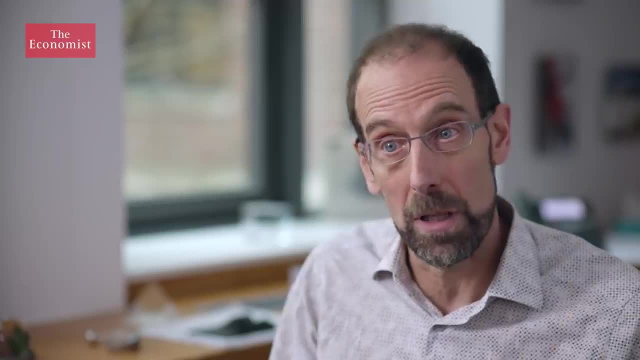 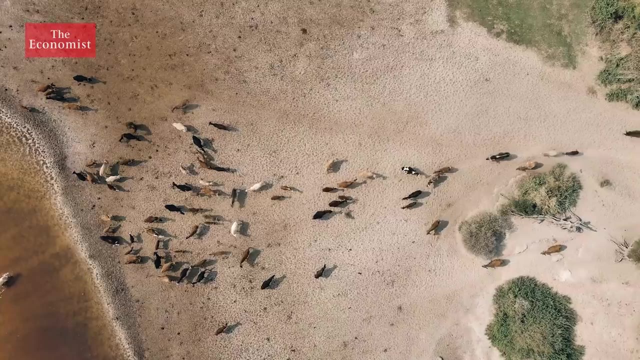 My view is it's a point of view with its own ethical implications, because the benefits of solar geoengineering would most be felt by poor people in hot countries, because you'd reduce those peak temperatures that are very destructive. Like most geoengineers, there's a lot of room for improvement. 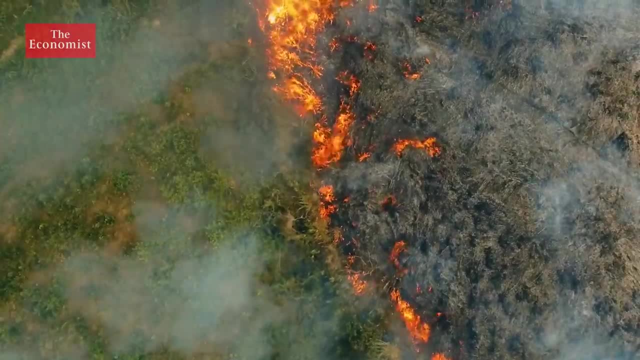 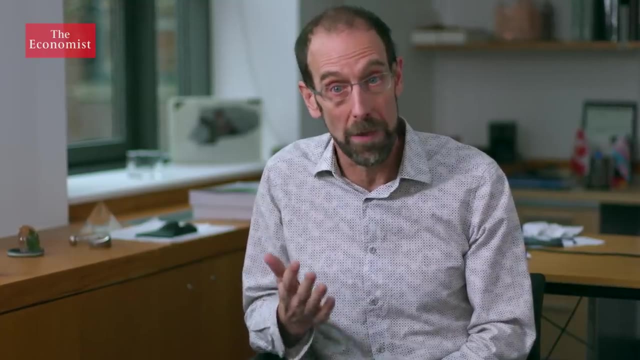 But there's also a lot of room for improvement. And there's a lot of room for improvement. I think there's a certain kind of monomania that we can only talk about one thing. I just don't think that's ethical or good public policy. 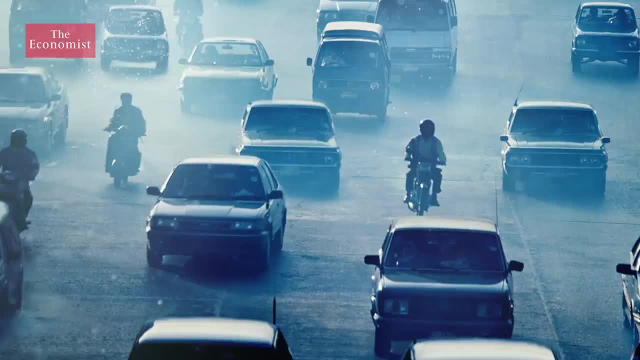 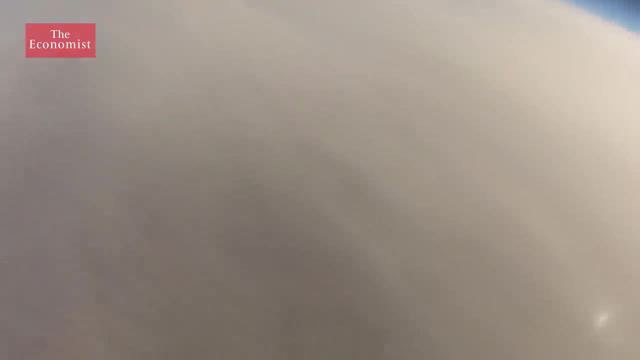 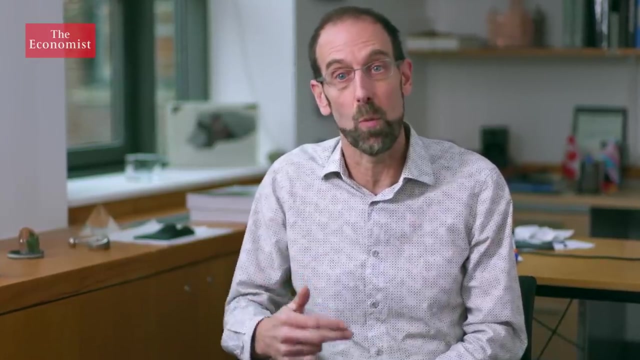 Of course we have to cut emissions, But that can't be all that climate policy comprises. He argues that stifling research into solar geoengineering now could increase the risk of negative consequences in the future. What blocking research does is it means that when the decisions about deployment 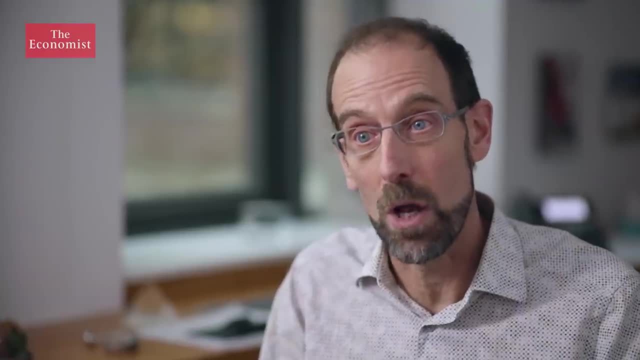 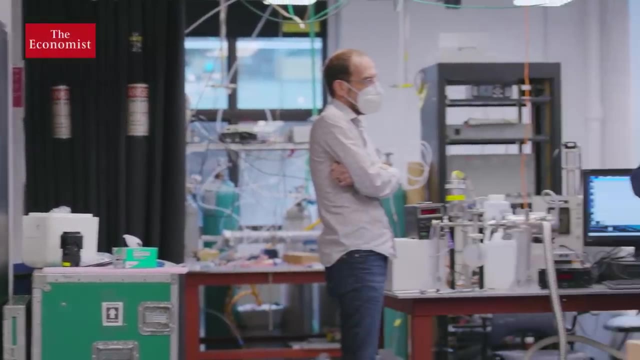 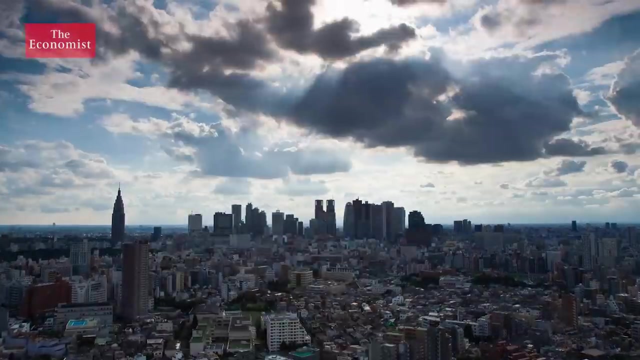 come onto the agenda, whenever that is, people will make that with less knowledge about the side effects, less knowledge of how to do this in a way that might be more effective, and probably with less serious discussion about how to govern it. Some studies have suggested that solar geoengineering, deployed equitably, 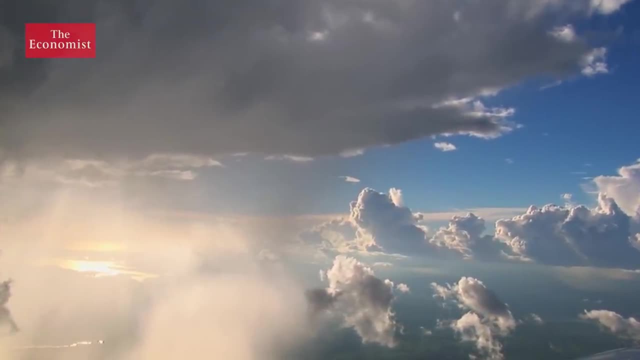 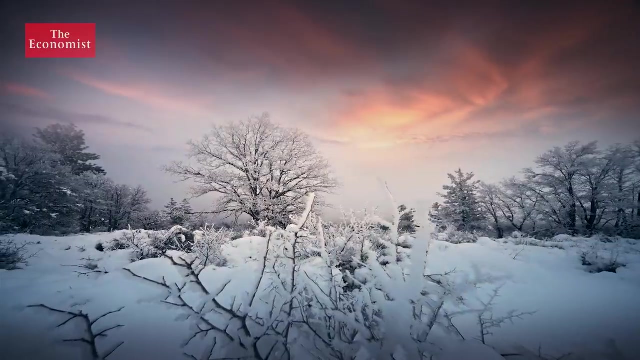 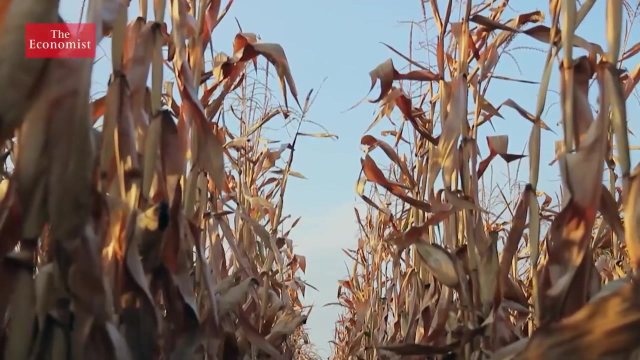 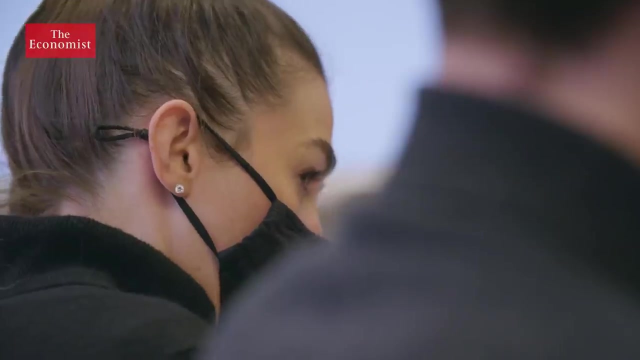 could provide climate benefits to all countries, But without global cooperation, technology designed to cool the climate could instead stoke international conflict. Because solar geoengineering could disrupt rainfall patterns and increase droughts, some countries may lose out. What happens if you dim the sun by geoengineering? 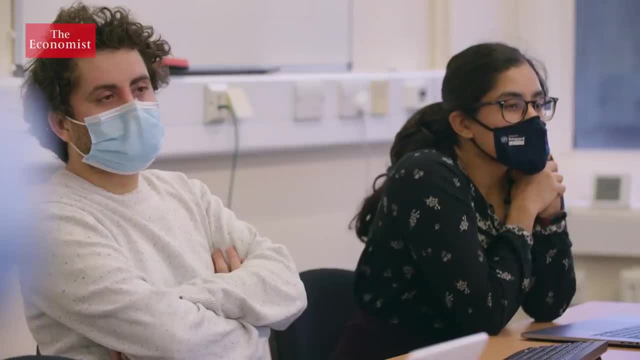 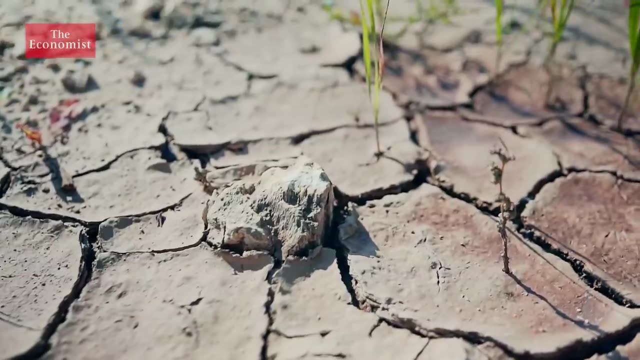 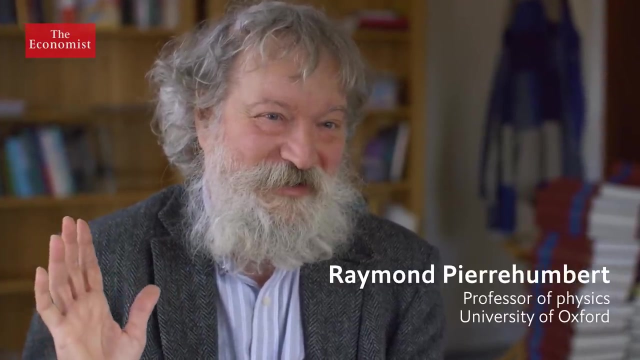 and remove solar energy from the surface. Scientists such as Raymond Pierre-Humbert believe a technology aimed at countering one global problem could create others, By ramping up disputes and sparking new ones. What if Russia likes an ice-free Arctic and wants less solar geoengineering? 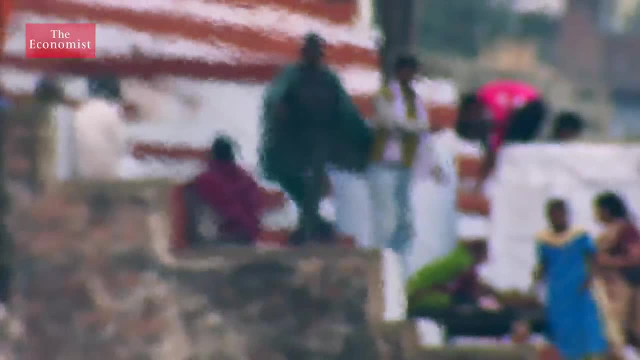 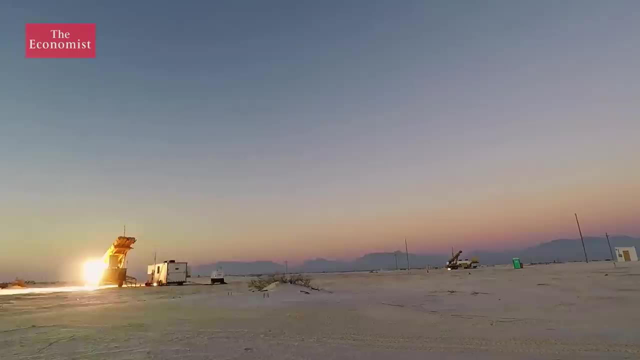 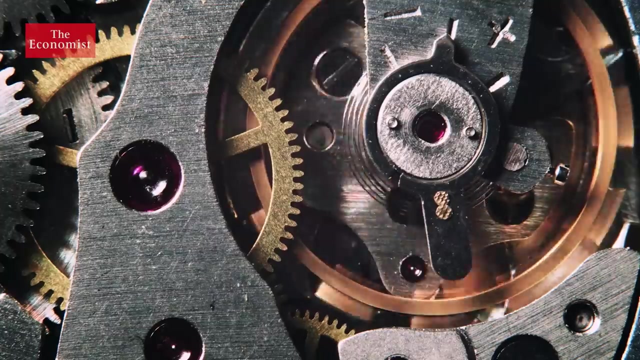 But what if India is laboring under killer heat waves so often that they really want to chill their climate down? Anything that increases the level of international tension in a world where nuclear arms are already proliferating is going to be a threat multiplier. Some also fear being locked into solar geoengineering. 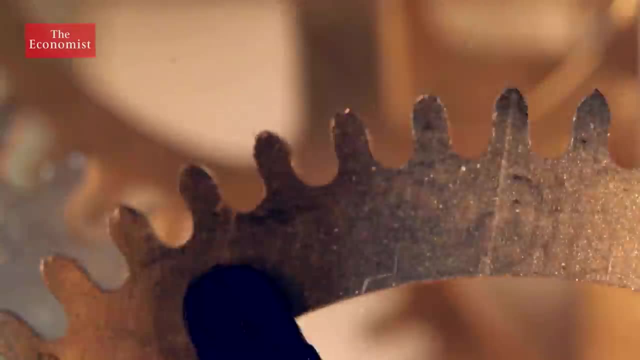 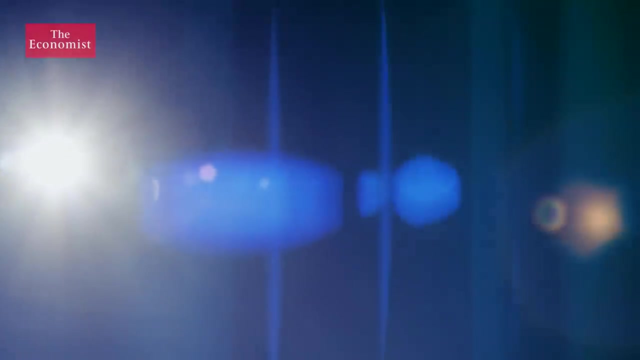 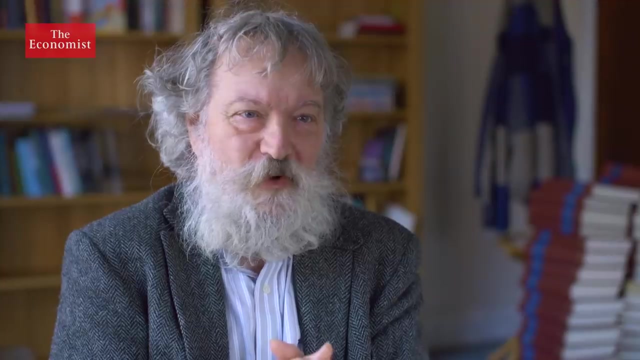 without any reverse gear. If humans fail to reduce emissions and rely on solar geoengineering alone, it could mean having to do it forever. In the worst-case scenario, stopping it abruptly could bring a disastrous termination shock- The word is terror, If anything forces the solar geoengineering to stop. 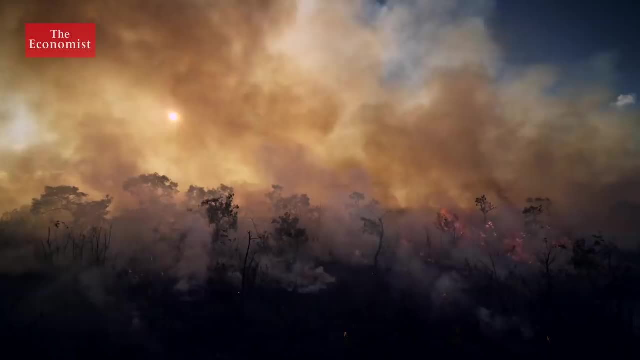 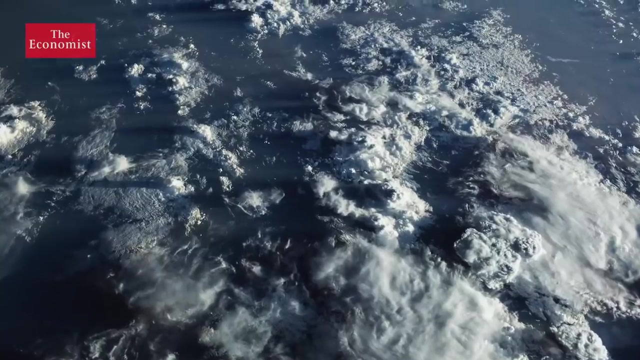 we're hit with catastrophic warming. It would be like living underneath a 100-ton boulder, just perched over the ocean Over your head, ready to fall at any time. Some scientists advocating research into solar geoengineering argue that termination shock could be avoided. 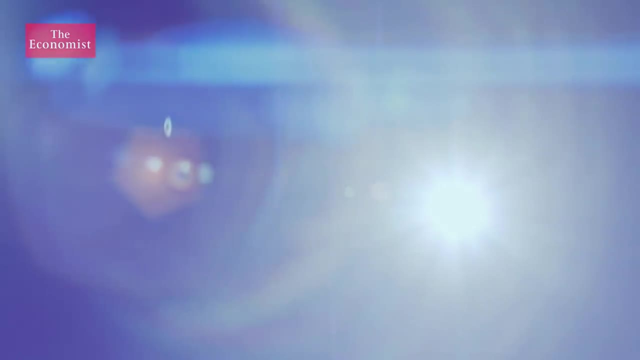 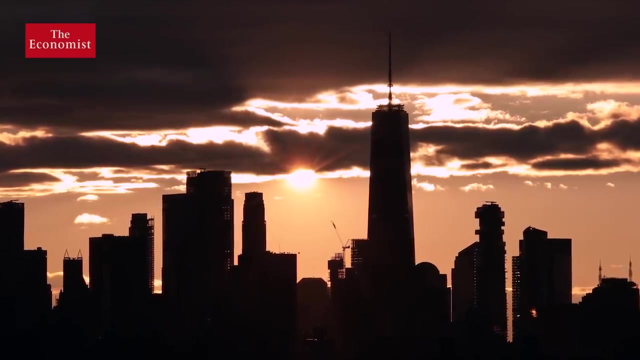 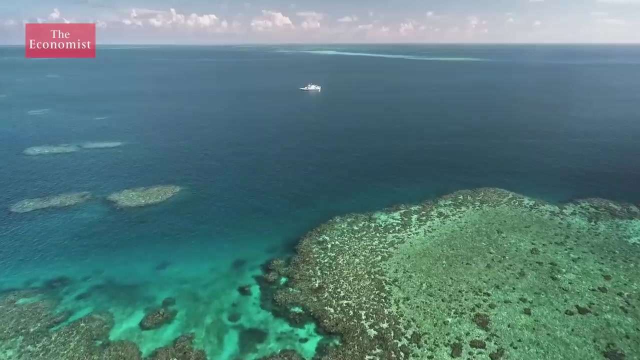 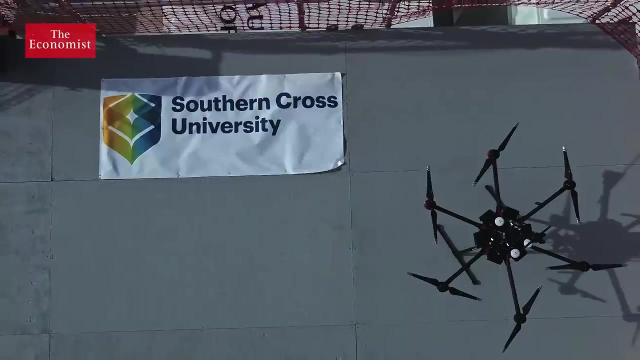 by gradually winding it down over decades. But would thinking less globally and more locally about solar geoengineering help to balance some of the risks associated with it? On the Great Barrier Reef, a group of scientists led by oceanographer Daniel Harrison are doing just that. 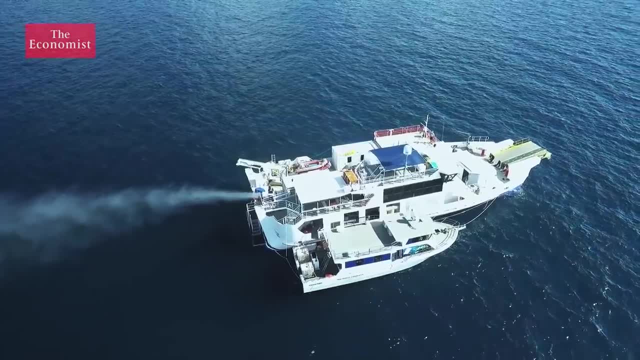 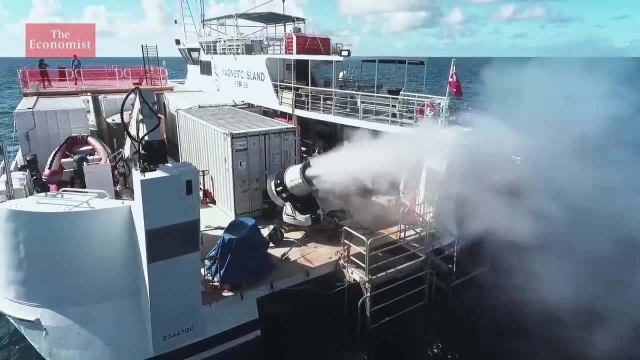 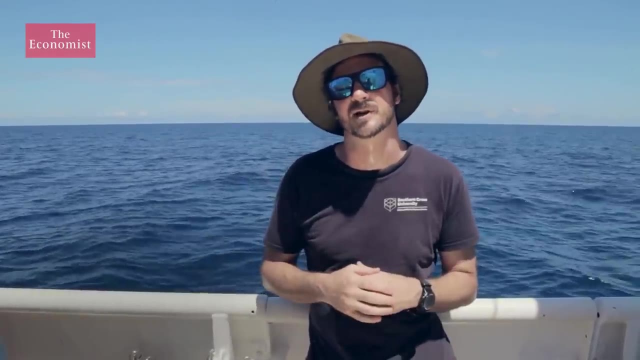 They're testing a kind of solar geoengineering called marine cloud brightening, The first time it has been tried outside of a laboratory. Cloud brightening is one of the ideas that, if it scales up how we hope that it may, it is potentially usable over the entire reef. 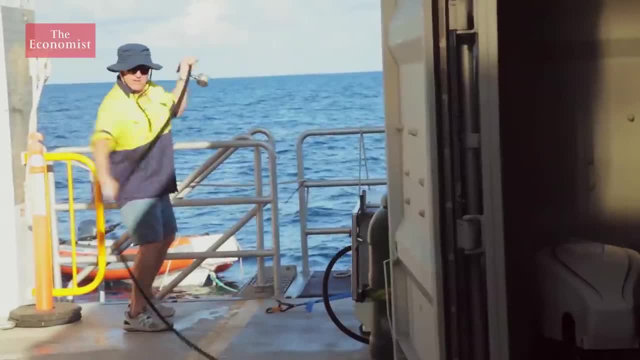 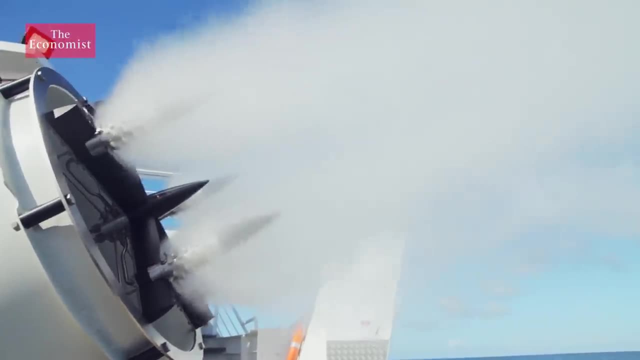 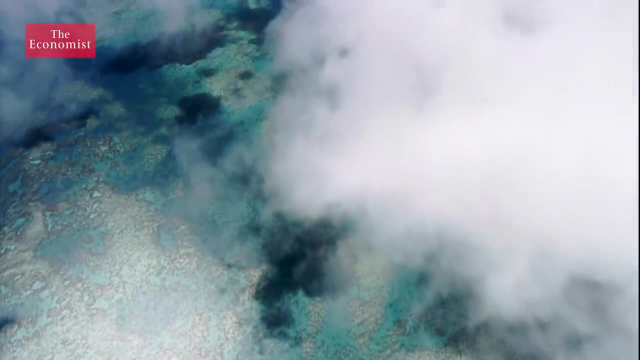 and can help all of the coral and all of the ecosystem. Using a custom-designed turbine with 320 nozzles, they release a cloud of trillions of nano-sized seawater droplets above the ocean, If the droplets can reach the clouds above. 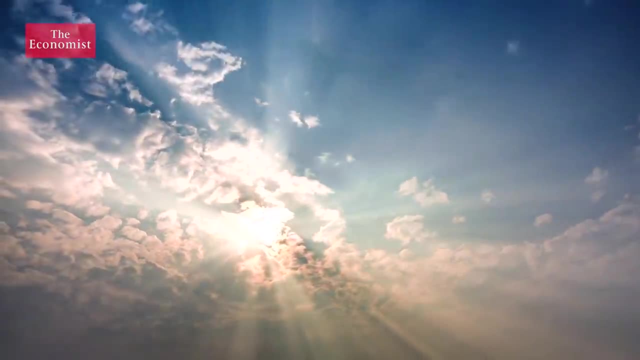 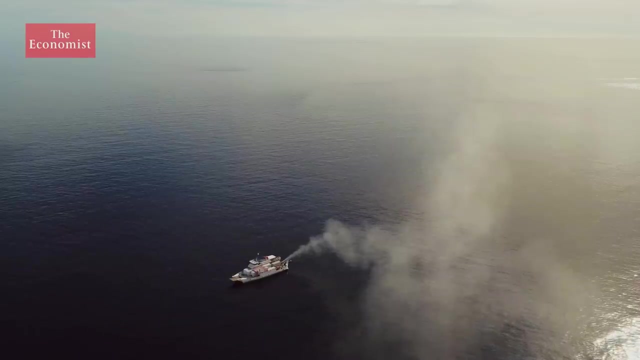 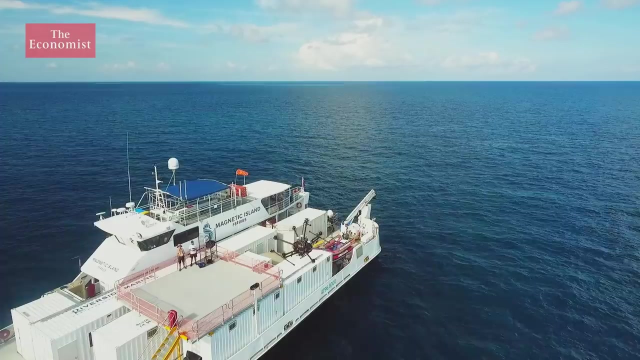 the theory goes that they will make them more reflective. What we're really interested in looking at is the behavior of that plume of sea salt droplets as it drifts away from the boat. We have a big focus on using drones as sampling platforms. 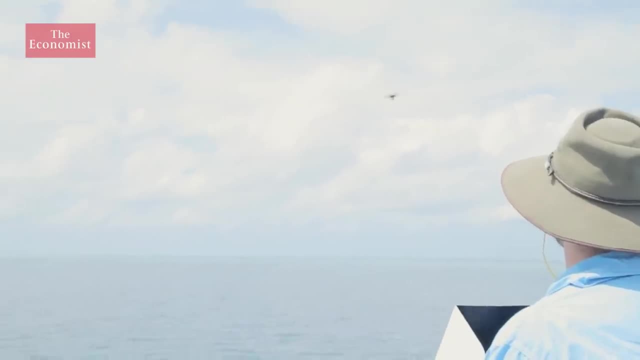 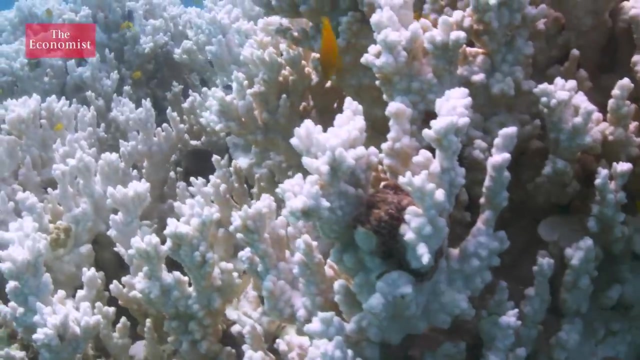 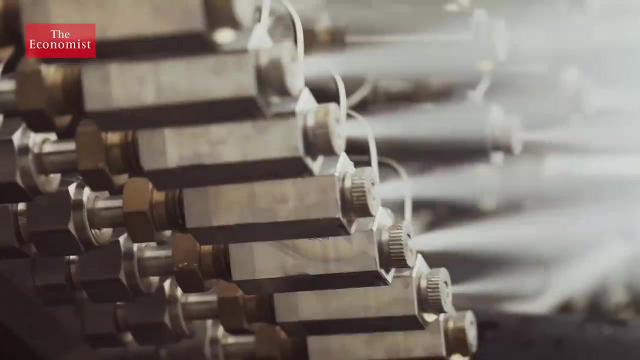 to measure the plume not just in a horizontal dimension, but also in a vertical dimension. If it works, the cooling effect could protect the reef from bleaching damage done to the coral during heat waves. Dr Harrison's vision for marine cloud brightening. 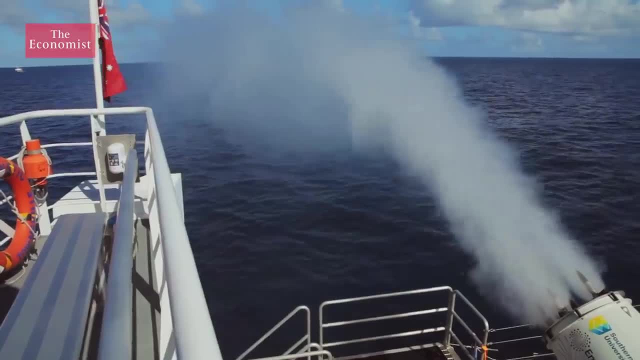 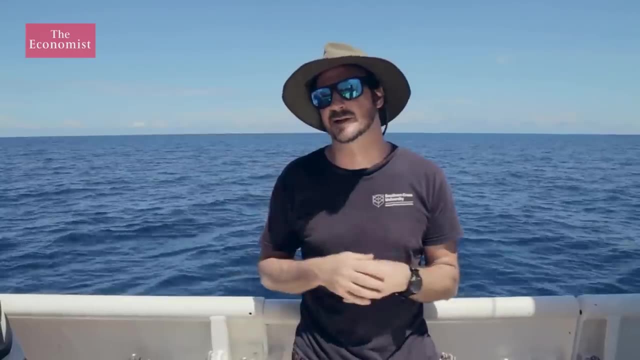 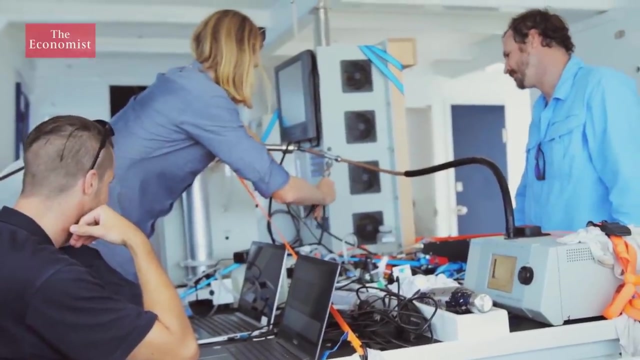 is targeted and temporary rather than an attempt to alter the climate on a larger scale. One of the great advantages of the cloud brightening concept applied regionally is that, in the very low chance that there were some unexpected or undesirable consequences, you could stop producing the sea salt spray.